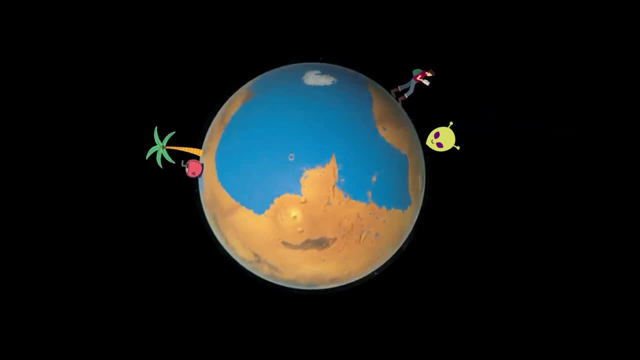 convey the position to you. if there is no common coordinate frame of reference that both of you understand, How will you reach another location when you have no clue where you are with respect to that location? Here's one solution. Imagine a pair of coordinates like the latitudes and the. 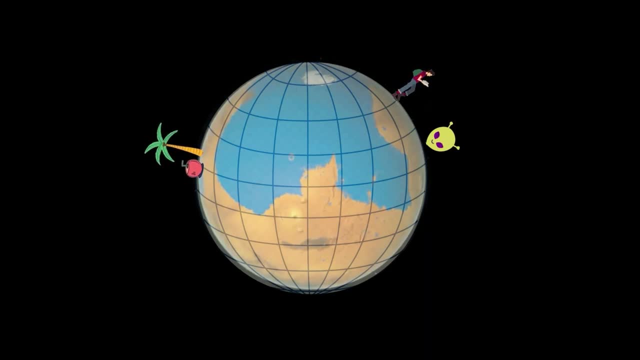 longitudes we have on earth. Now, based on this frame of reference, you not only know where you are on the planet, but also the relative position between you and the food. This is localization, the knowledge of your poles and orientation with respect to the world, or the map coordinate system. 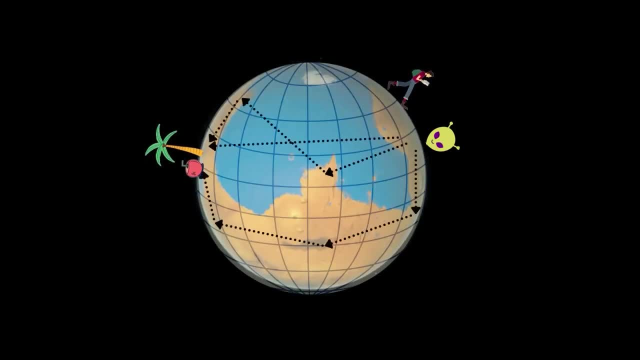 Now there's still one more problem. You cannot directly see the food, So you don't know how to form a path from where you are to the food location. Yes, of course you could randomly start moving in the direction of the food and try to avoid obstacles on the way. However, reactive navigation. 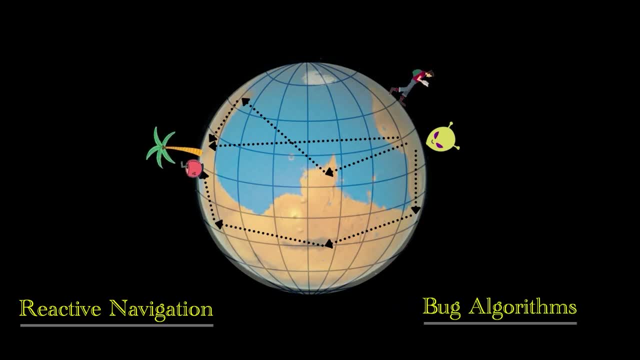 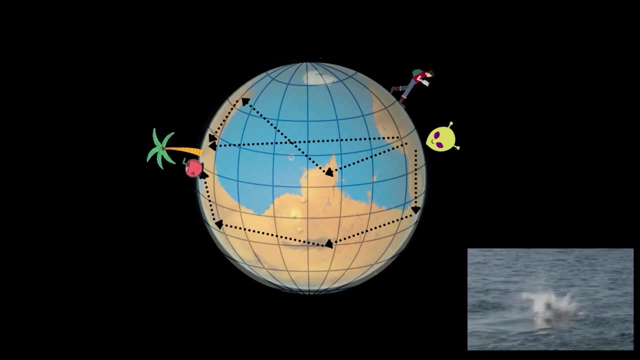 or bug. algorithms of this kind has several disadvantages and unpredictable conditions. You could get trapped in the food. You could get trapped in the food, You could get trapped in the several areas or even fall in the sea. Hence, in autonomous robotic systems, it's best to pre-plan. 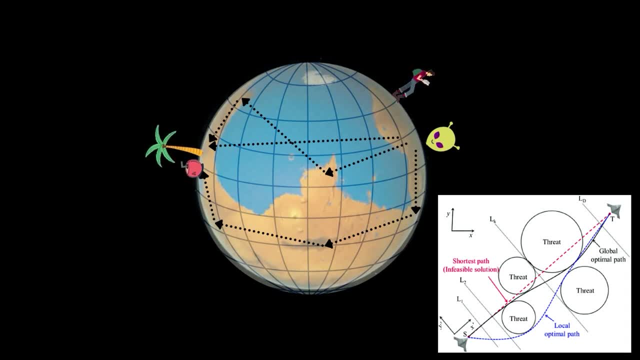 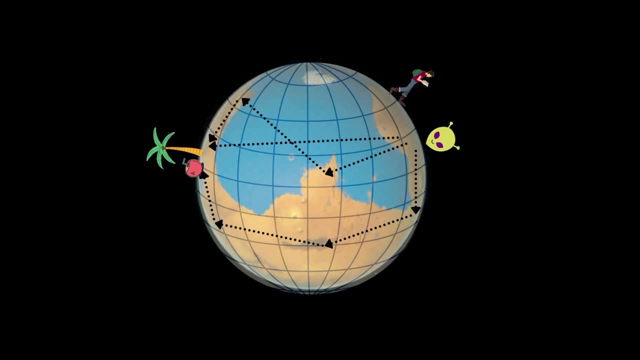 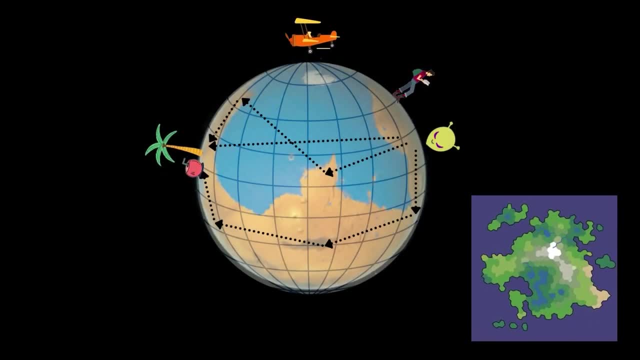 need to have a computer. You'll need to have a computer. You'll need to have a computer. Rather, while you're planning and planning to capture a complete tool of the world, while simultaneously being aware of your location, you will be able to create a map with the information that 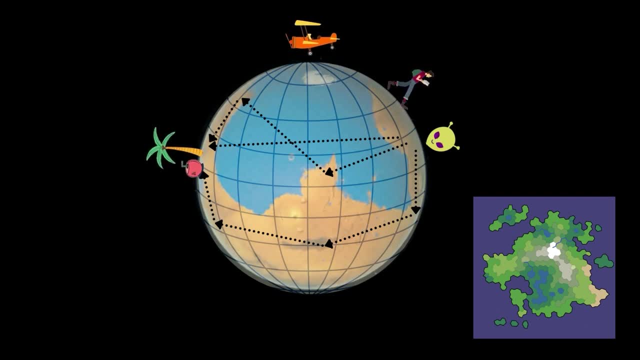 you perceive using your senses and save the build map of the imaged in your mind for future path planning and navigation. This is called mapping And once you have this map or an occupancy grid, distinguishing between obstacles or verschiedenen goals or advantageous issues may become difficult for you to forgive and ignore. You may have the satisfaction to 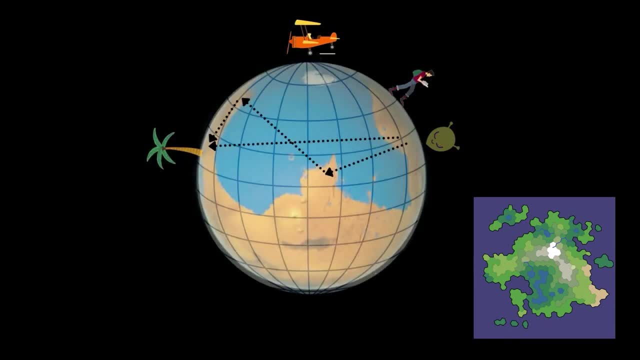 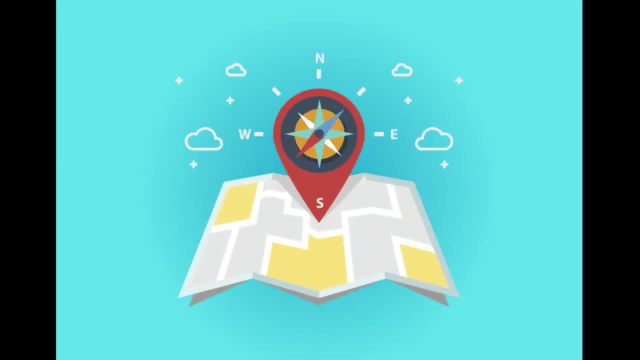 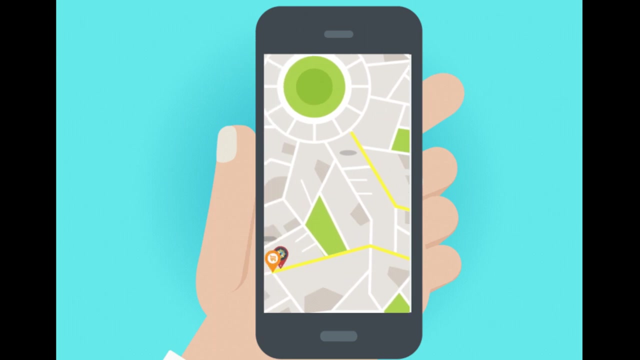 obstacles and the free spaces, you can now form an optimized path from any point A to point B. This is exactly how even GPS forms a path for you. It knows where you are, where you need to go, with a common frame of reference, and what the world looks like. 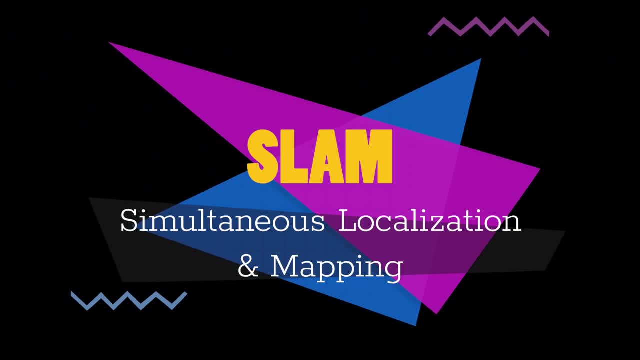 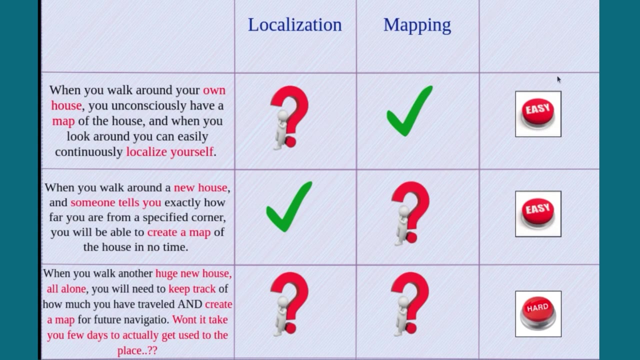 Now that you understand the importance of localization and mapping, let's answer a few questions about the game changer, SLAM, before we dive into understanding gmapping. So, firstly, why is SLAM considered a difficult process? Yes, it is because we are trying. 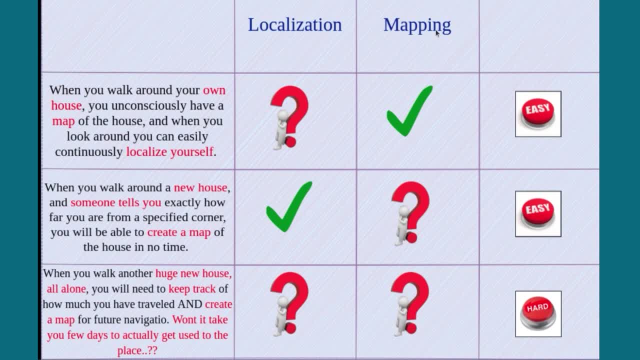 to perform two dependent tasks simultaneously and it becomes a chicken-egg problem. Let me put this in very simple terms. When you have a map, it is easy for you to look around for features, landmarks, etc. On the other hand, when you are localized, you can create a map of the surroundings and 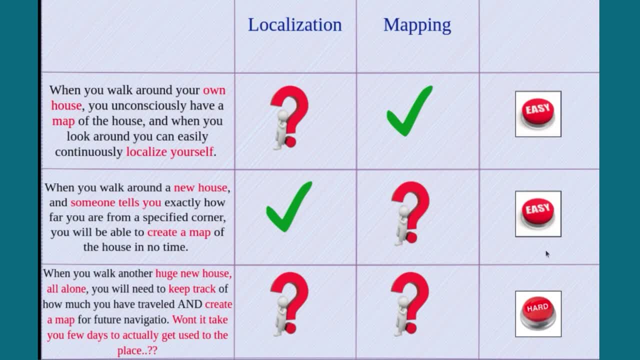 storing what you see as a 3D or spatial model. However, when you neither know where you are nor what the world looks like, it becomes a very challenging task, because now you are completely relying on probability, distributions, uncertainties and estimation, which can broadly 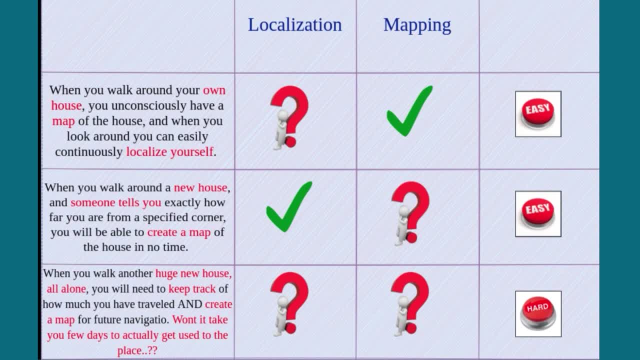 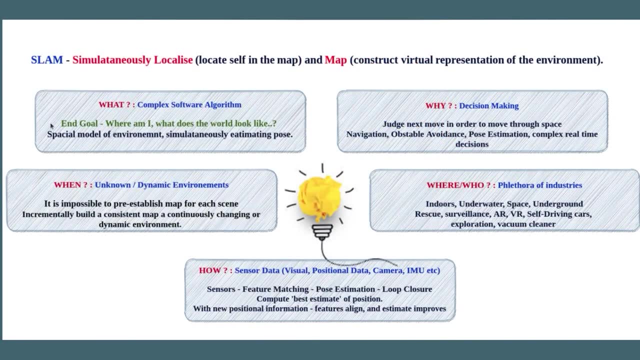 get affected by different parameters. Hence, a robot needs a smart, complex brain like ours, And that's the SLAM algorithm, where the end goal is very simple: You need to know what the world looks like and where you are in it. 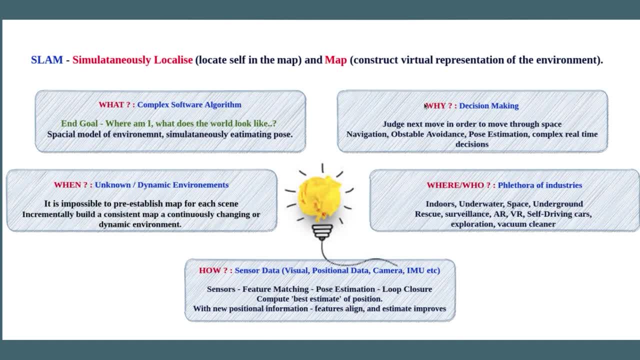 Why is it needed? As we already know, it is essential for a robot to not just navigate autonomously and avoid obstacles, but also take critical decisions and perform tasks efficiently and safely. And one of the most important questions is: how do we achieve SLAM, The very first step? 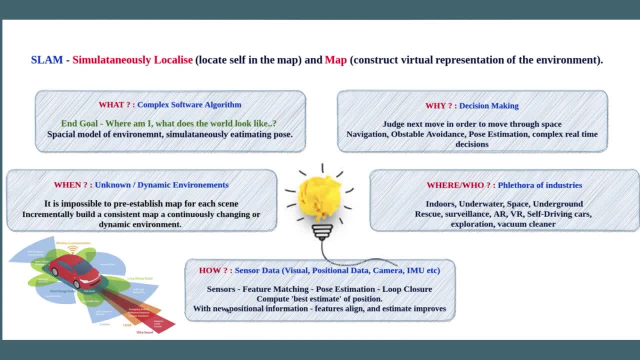 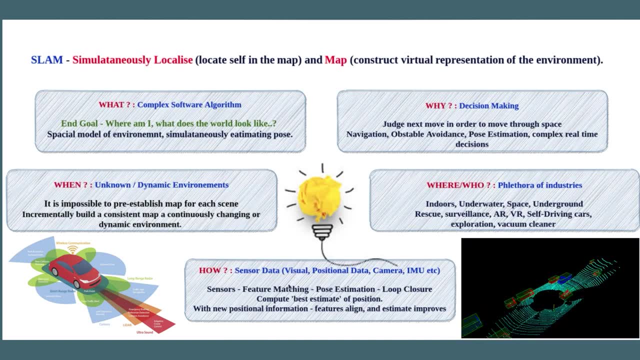 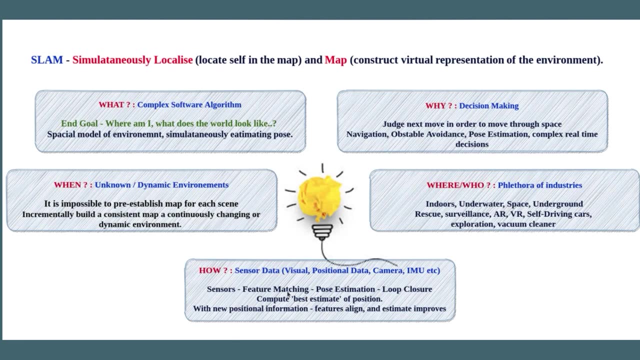 in SLAM is to gather appropriate information using the right sensors for the right application. We then use several techniques, such as Kalman filter, to fuse the data together, after which it is a multi-step process where we perform feature matching, pose estimation and loop. 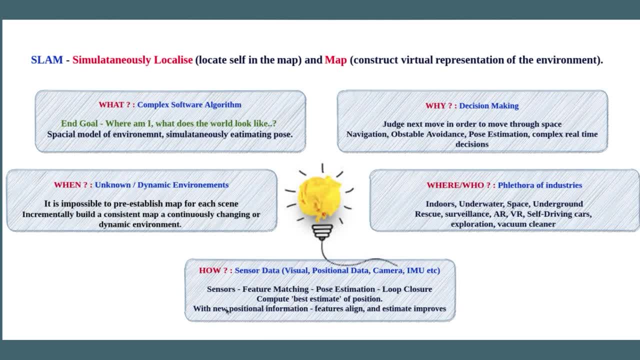 closure. And it's important to note that SLAM is a multi-step process where we perform feature matching, pose estimation and loop closure. And it's important to note that SLAM is a multi-step process where we perform feature matching, pose estimation and loop closure.